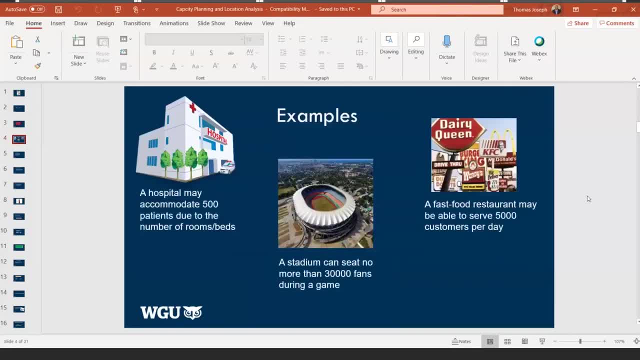 So some examples we can look at. we could say a hospital, for example, may be able to accommodate- what about 500 patients? That's based on the number of patients, The number of beds that it has or the number of rooms that it has, the accommodation. the maximum that it can be accommodated, the maximum number of patients this hospital can have is 500. Not about 500, but 500. And that's based on number of rooms and or number of beds. 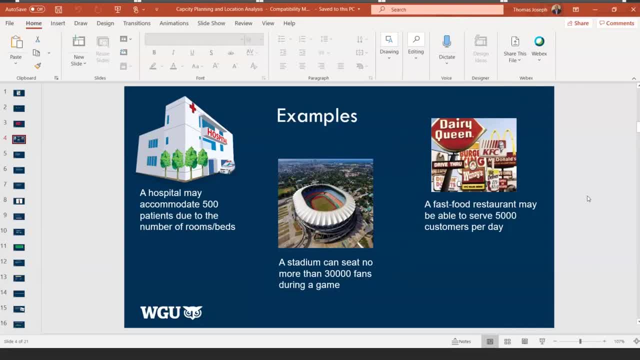 Another example: if you think of a stadium for those of you who like sports- you go to sports activities such as football games or basketball- A stadium can seat no more than 30,000 fans during a game. That would be the maximum capacity. 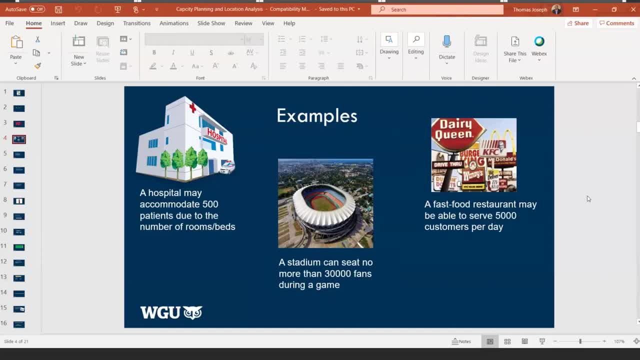 And another example. we could think of a fast food restaurant able to serve, let's say, 5,000 customers per day. That's the maximum. You cannot do any more than that. Think about another example. if we just kind of get something off the top of your head, 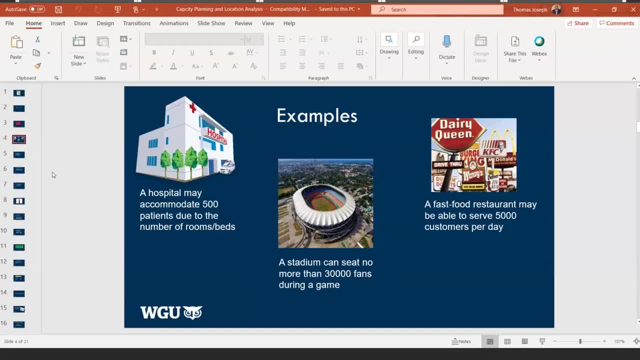 If you look at the speedometer of your car, no matter what car it is, it's going to be the same speed as your car. So let's say you're in a car and you drive. There is that number. it shows that says some of you might be 240 miles per hour. 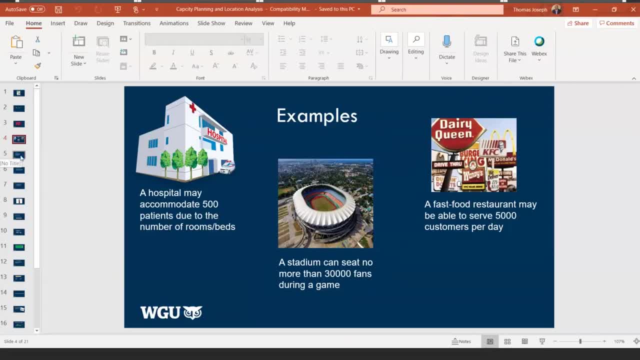 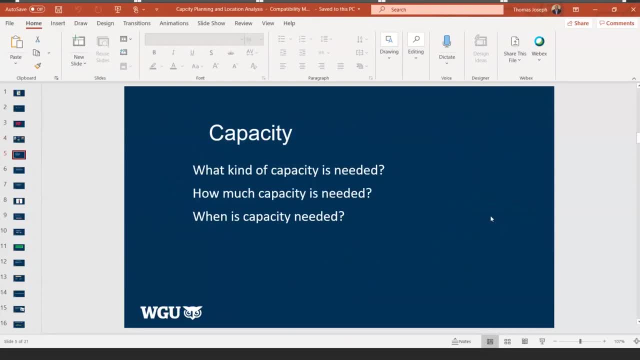 So that would be the maximum speed that the car can go Right. So that is, what capacity is the maximum output? So when we think of capacity, there are certain questions that come to mind. Number one: we have to think of what kind of capacity is needed, right, 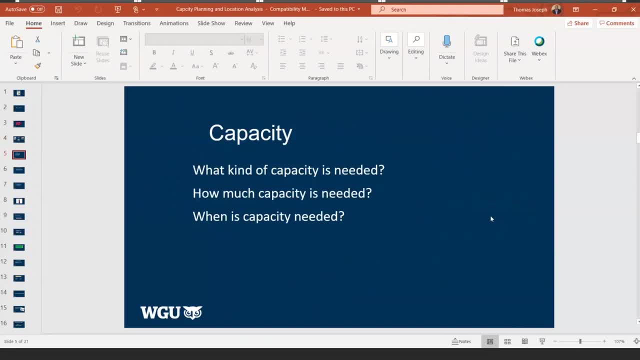 What kind do I need? um, how much capacity do i need, or how much capacity do the organization does the organization need? and then another question that can be asked when we think about capacity is: when is capacity needed? so these are the three main questions that we ask, and these are things that we do. 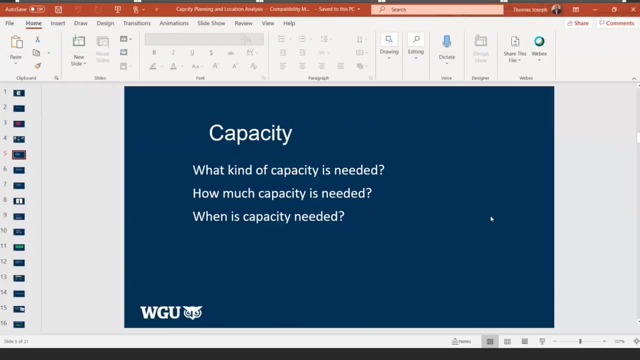 in our lives. so let's think about it. if you are a single person, um, and you you know, enjoying life, having a good time- you more than likely will have, let's say, a one bedroom apartment, because it's me alone, i don't need more than that one bedroom apartment. 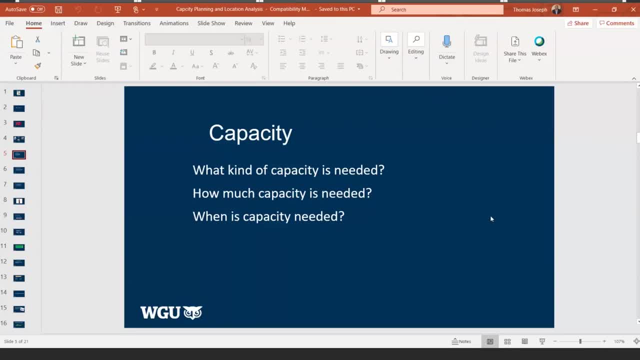 that is the capacity that i need. so let's take, for instance, you decide, okay, i get married and then i have kids. now that i have two, three kids, what do i do next? right, then i will need: where do i put the rest of my kids? where am i going to put my kids? 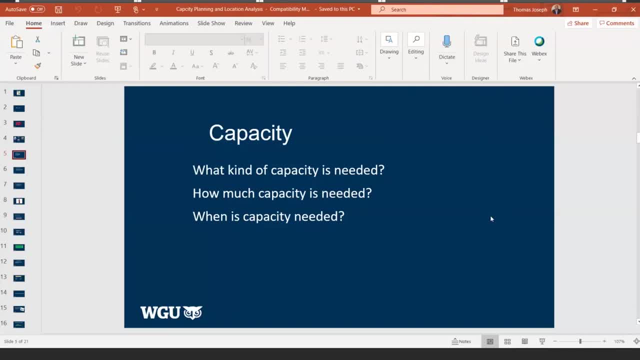 they can't sleep in the bed with my, my spouse and i. we have to find room for them. how much capacity we need. if i have three kids and my spouse and myself, then i need much more capacity. how much is needed and when is the capacity needed now that we have three kids? 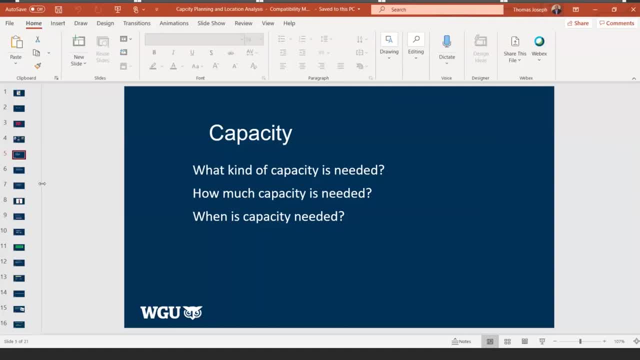 we have to find us more space to live. the same thing happens with business. they make that same decision, we do it every day in our lives, and then businesses do the very same thing as well. let's talk a little bit about measuring capacity. again, if you take the example that we use- and it's i try- 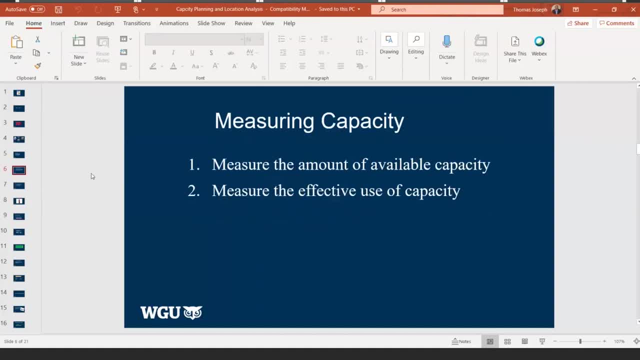 i try in my teachings i tend to focus a lot of those concepts into more practical perspectives, because i believe if we can understand those prospect concepts from practical, applicable, day-to-day terms, then it becomes easier for us to see how this applies to healthcare, how it applies to any industry that you are. 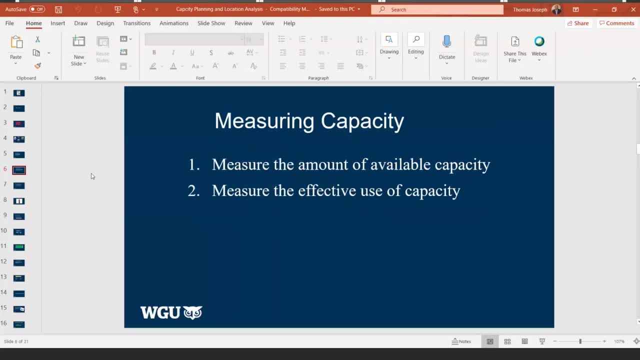 in right, no matter what it is any servicing manufacturing production company that you're in, because the concepts apply the very same way. so when we think of measuring capacity- because remember the thing about operations management, it's all about measuring things- efficiency- you have to measure how well you're doing. 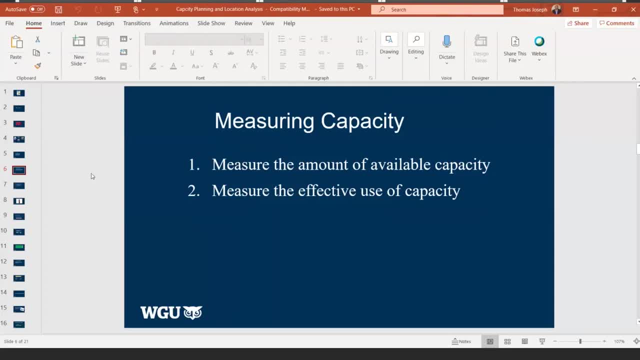 right, in order for you to know how well you're doing. so it's all concerned about efficiency and customer satisfaction, but in order for us to know how efficient we're doing as an organization, we have to measure somehow everything that we do. so there is the measurement. it can measure the amount of available. 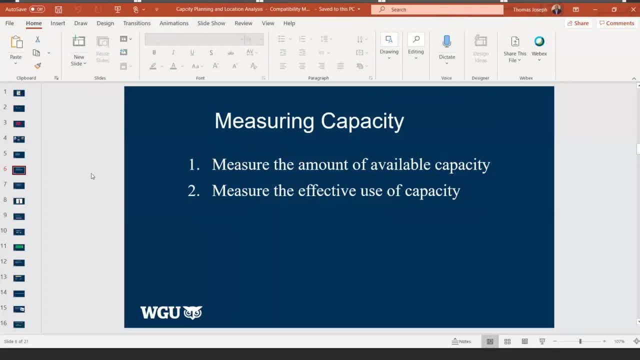 capacity. and number two, the organization can measure the effective use of its capacity. so we have to be able to know, as an organization, the amount of capacity we have available. again, if we take back our example as a family, we have to know how much capacity we have, measure the amount we have. one bedroom. 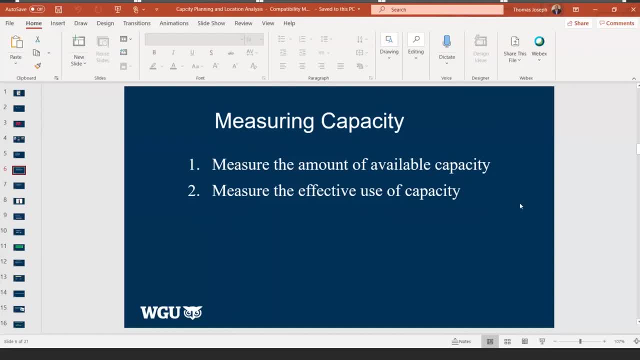 we have three kids and a spouse and and two spouse right- a husband and a wife or whatever spouse relationship we have right. and then we have to measure the effective. how effective are we using that? so let's first of all talk about the amount of available capacity. how do we measure that? 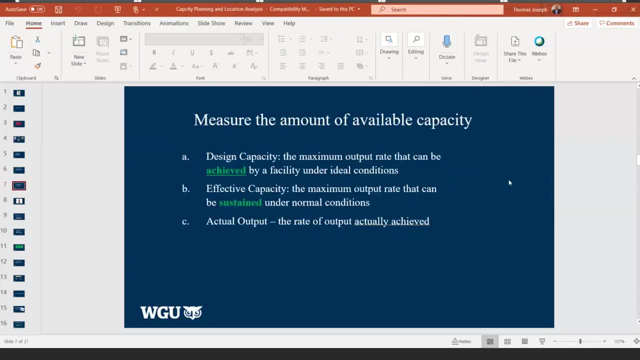 so two concepts that come into play, or three, but more precisely two. we think about design capacity. again, design capacity is almost definitive as capacity itself. when we talk about regular capacity, and which one is the good one? is it taking off or it's about what is capacity? 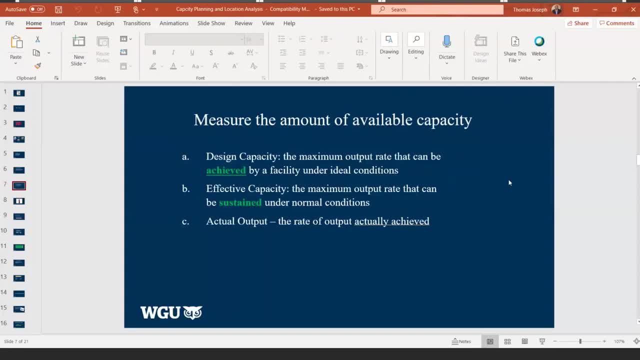 Design. capacity is really the maximum output rate that can be achieved by a facility on the ideal conditions. So if things are going well, like, we have a stadium that can seat 30,000 people. so that's the design. That's what it was designed to accommodate. 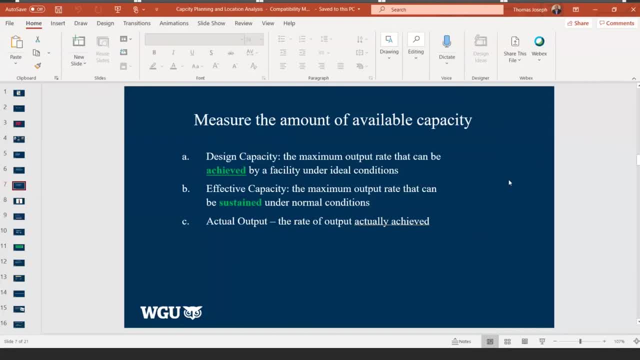 That's what it was designed to see. I don't know how many of you guys have walked into a building and you see the sign that shows maximum capacity: 500, right, Something like that. And then it's ordered by the sheriff department. 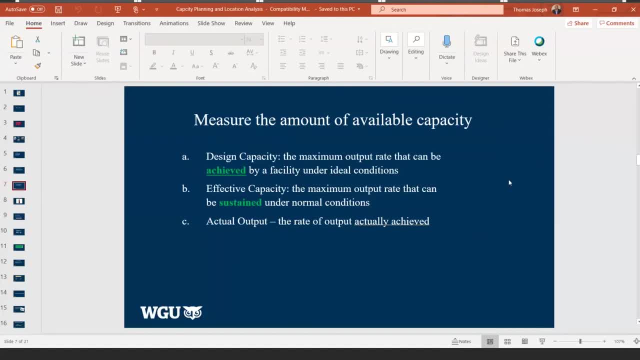 and stuff like that. So that's what it's designed for, That's what your design is. But remember, on the ideal conditions is critical. Out of the design capacity, we have the concept of effective capacity. Effective capacity less than design capacity. 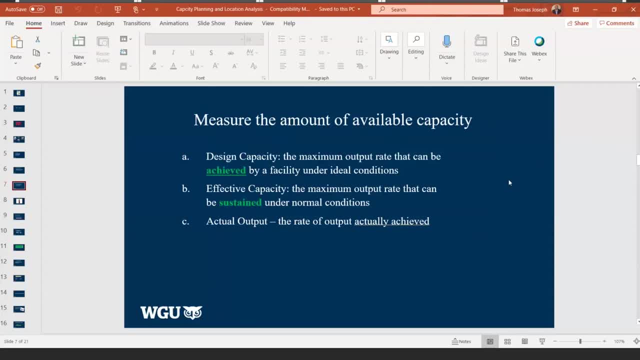 It represents the maximum output rate that can be sustained. Right Design capacity achieved, effective capacity sustained on the normal conditions. So think about it. I always look at it this way If I have a car that's designed to go 120 miles per hour. 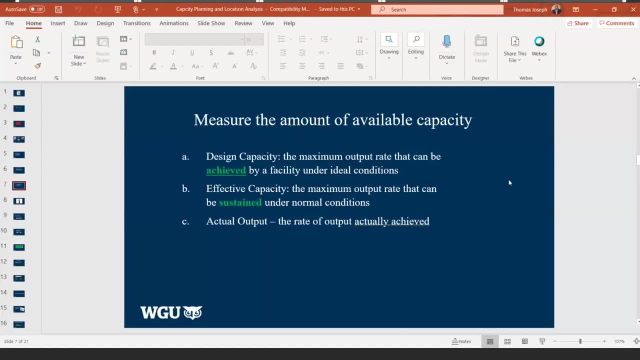 I decide 120 miles per hour. That's the maximum. That's what it was designed to go. I decided that I'm going on a road trip. It's going to be highway all the way. The maximum speed on the highway. highway has the signed speed limit: 70 miles per hour. right, I can drive that effective capacity. 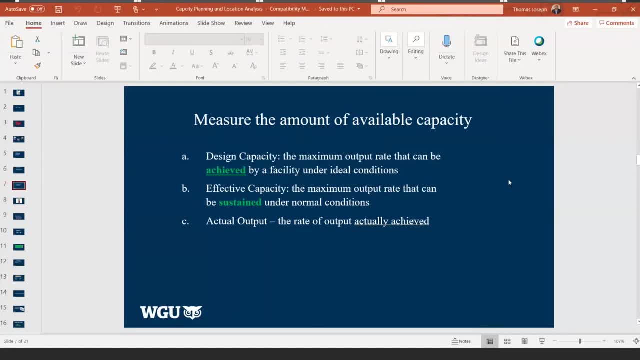 of 70 or 75 miles an hour. put my car in cruise control, that's normal conditions. I will get to where I'm going in X amount of time, right. But the third aspect we have there is actual output. That's the rate of output actually achieved. Did I drive from point A to point Z at 70 miles an hour? 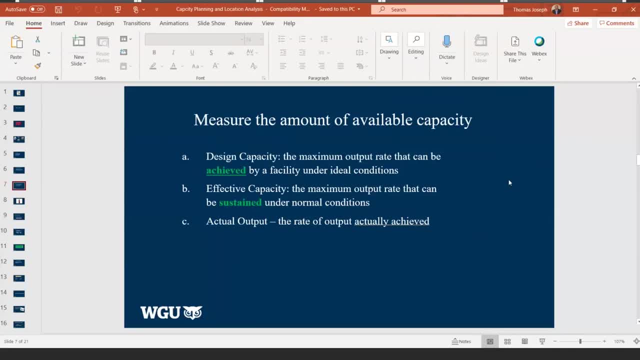 all the time. No, Maybe I run into some traffic, have to turn off my cruise control and all of that good stuff. So three things: when we measure capacity, or the available capacity, we look at design capacity, how much we can achieve. do we have effective capacity? how much can we sustain? 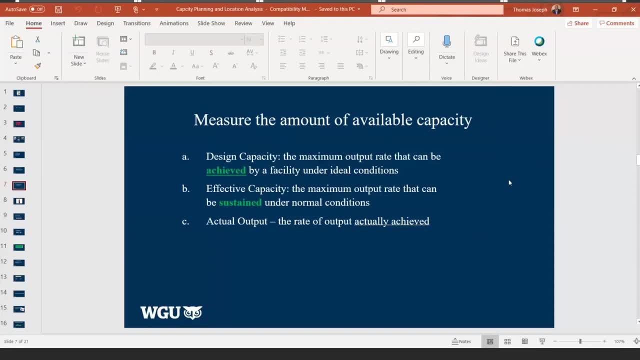 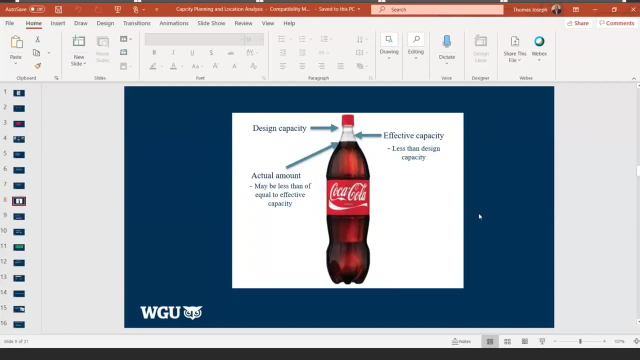 can we keep up with that rate Right, And then we have the actual output, which is exactly what we achieve. So here is an example of a Coke bottle. This is what capacity, plant design, capacity, effective capacity and actual capacity would look like. So the bottle, all the way to the top, that's what it's designed to take. 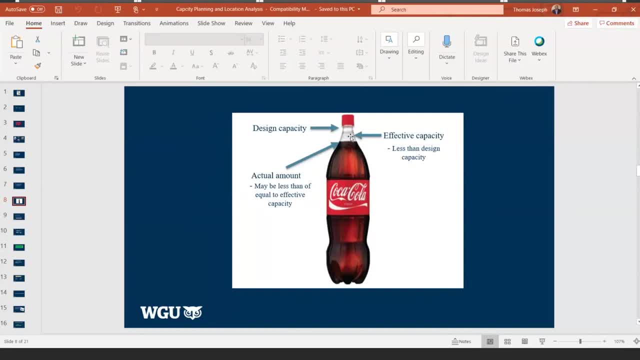 The effective capacity. that's probably where okay, if the bottle is at that level, then we could say, yeah, I got me a good Coke bottle, right, I got a little more than I thought. And then the actual capacity. 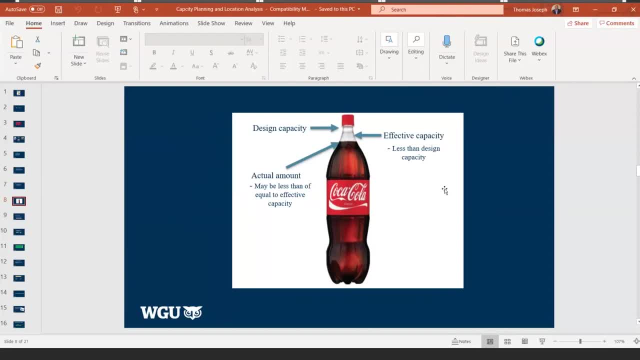 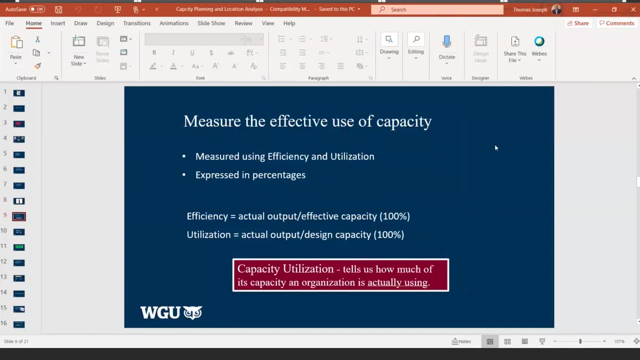 capacity is generally can be less than effective capacity as well. So when we think so, that's measuring the availability of capacity, how much capacity we have available. Another aspect is to measure how effective we are using our capacity. So, for example, if, as a head nurse, you have 25, 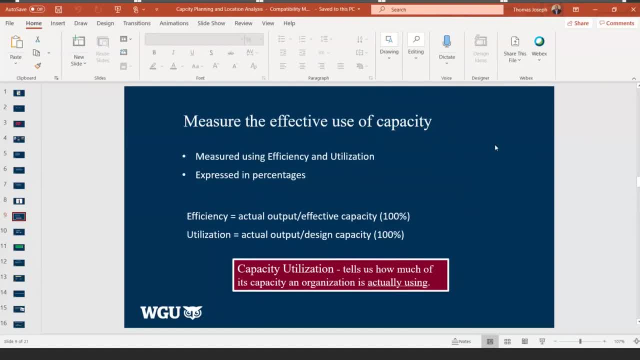 staff and then you have 100 patients for the night- right, I'm putting a lot there. Then it's important to measure the availability of capacity. So, when we think so, that's measuring the availability of capacity. So what I'm saying is it's important for you to know how effective am. 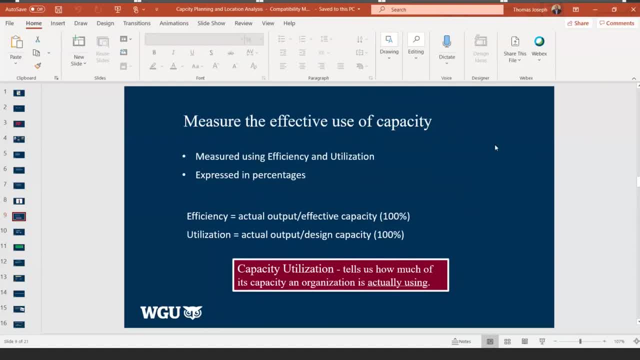 I using my nurses, my capacity, so that my patients are getting the type of treatment that they have. If you are unable, if it's your manager of any organization, a production plant or anything of that stuff, it's important for to know how effective are you using the space you. 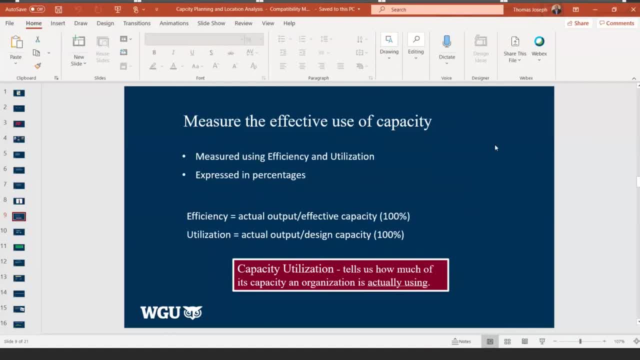 have available, but also, how effective are you using the employees that you have available so that you are getting the best out of them every day? all right, So when this happens, So when we think of measuring the effective use of capacity, we talk about measuring use and efficiency and utilization. 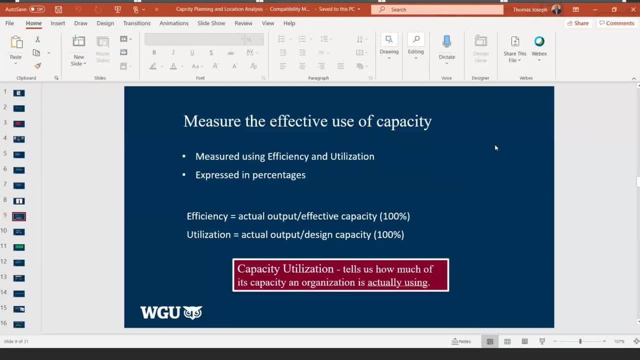 Both are expressed in percentage. Now I don't want you guys to get caught up in this math concept. This is not a math oriented course, so you will barely get any type of math questions on your exam. But just remember, when we think of measuring, this is measured in percentage. 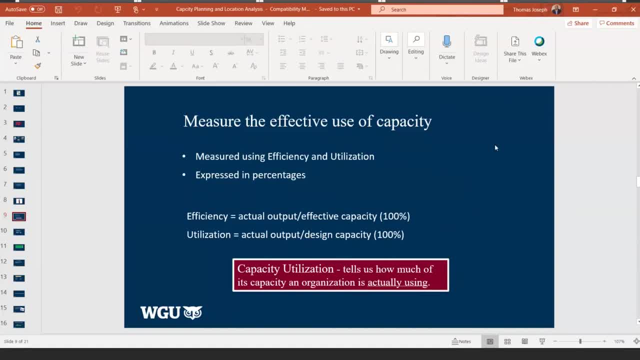 Efficiency is measured by dividing the actual output by the effective capacity, and then that's a percentage. Utilization calculates the actual output divided by the design capacity in a percentage form. Now here's a major one: Capacity utilization tells us how much of its capacity an organization is actually using. 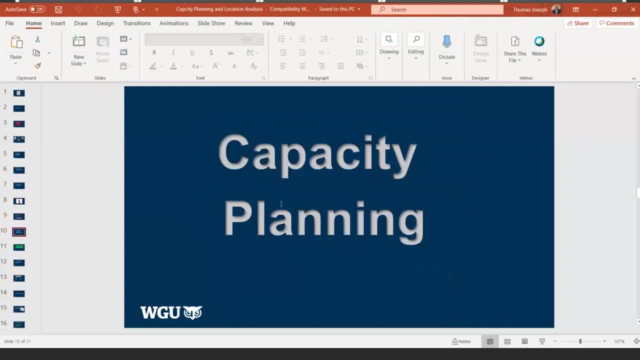 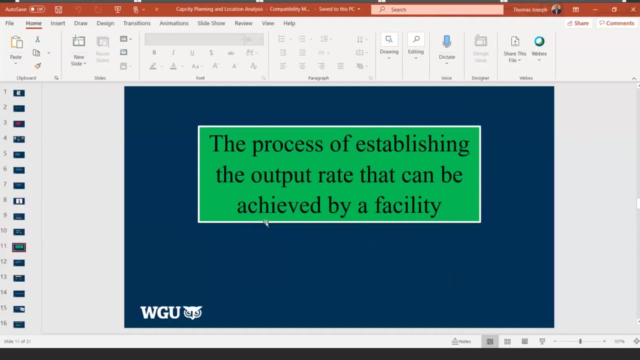 How much of the space that we use. So, now that we've created that background of what capacity is, the next step as a manager is now I have to decide: how am I going to plan my capacity? How am I going to take care of the space that I have and utilize it to its maximum use? 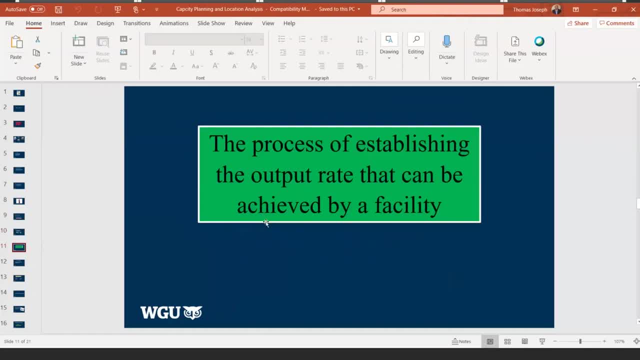 How am I going to utilize the employees that have been assigned to me and ensure that I am getting the most out of them? Not that I'm slaving them, but I am getting the most out of them. They're satisfied, they're happy, they're not burned out and overworked. 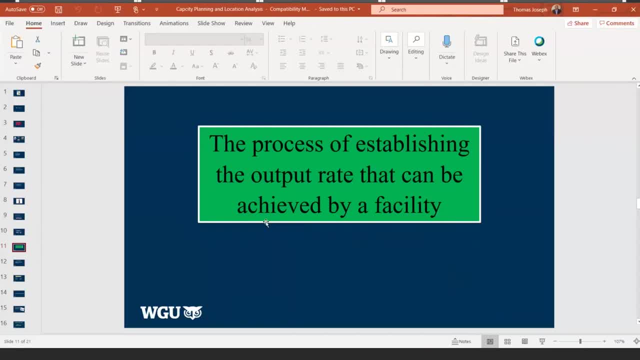 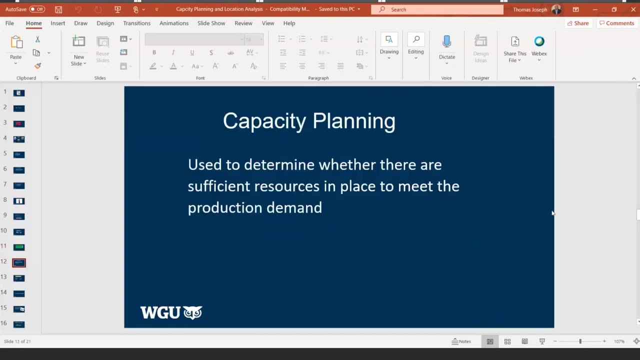 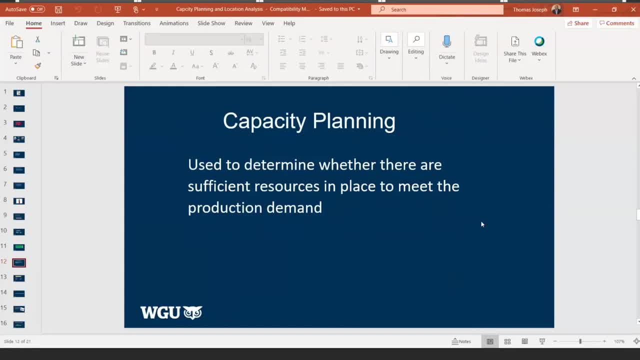 Capacity planning is used to determine whether there are sufficient resources in place to meet the production needs. Capacity planning is used to determine whether there are sufficient resources in place to meet the production needs. If we look at it from a healthcare, for example, standpoint, it could be whether there are sufficient resources- that would be medication, beds, right, the operating machines, all of those equipments and nurses- to meet the demand that we have, or production demand would be the patients that we are serving. 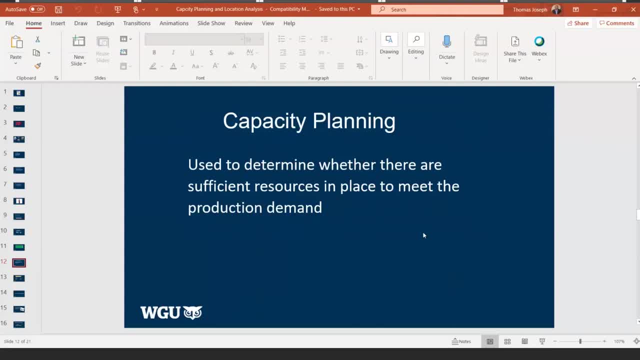 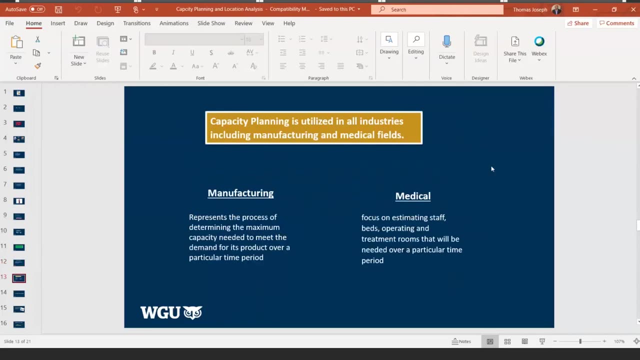 If you own a private practice- like, let's say, you own a CPA office or any of that sort- is: how much are you using the resources that you have to meet the demand of your customer? That's what capacity planning is all about. It is utilized in all industries, both for manufacturing and medical. From the medical standpoint, it's focused on estimating staff, beds, operating treatment rooms that will be needed over a particular time period. 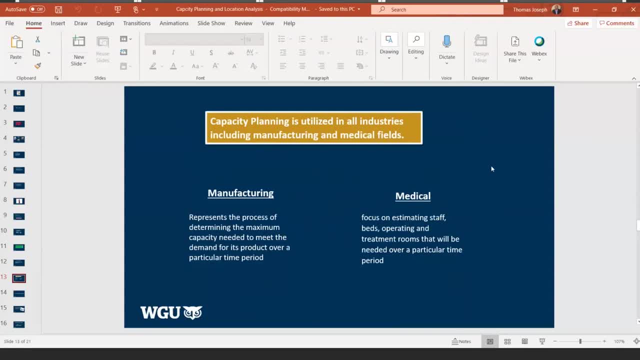 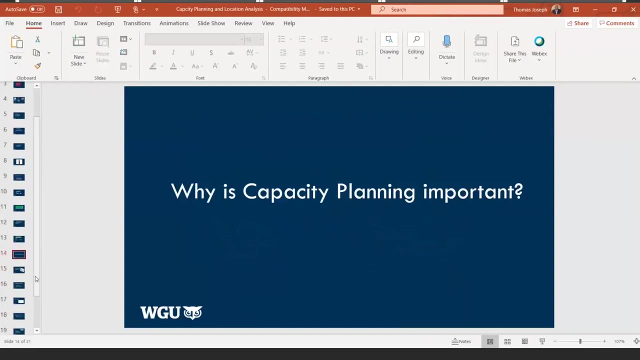 And manufacturing side. it represents the process of determining the maximum capacity to meet the demand for its products over a particular time period. So what do we get out of all of this? We're looking in perspective of maximizing what we have available, And I'm saying we because I want you guys to think from an operations manager's perspective. 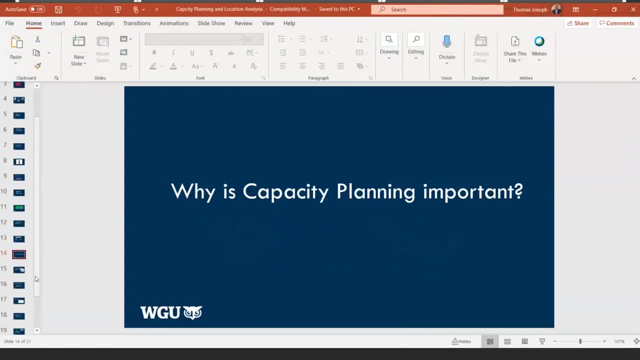 Think of it in terms of you functioning in the capacity of a managerial role within operations. Think of it in terms of you helping the organization and helping with the decision-making process, or you are looking through the lens of the manager or the CEO or head manager of your organization and be able to understand what is driving the decisions that they make. 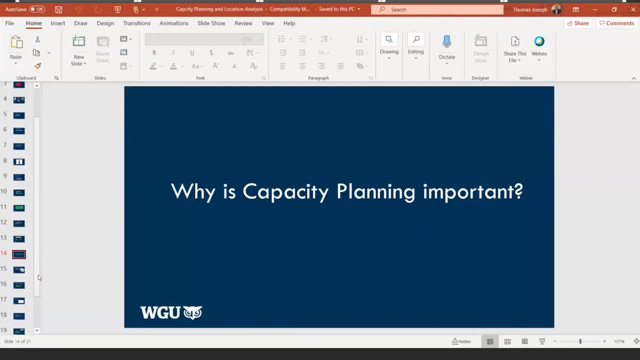 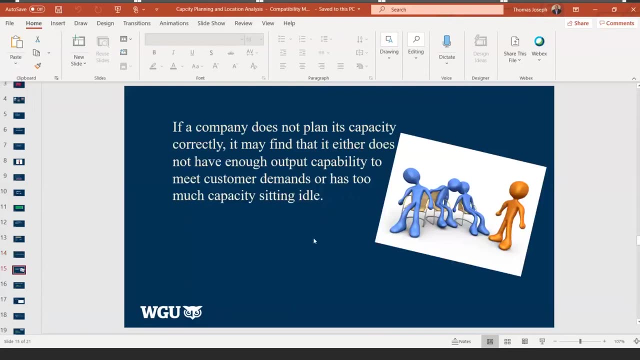 Why is it that I'm only assigned eight employees instead of 15?? Why am I assigned 15 employees instead of five? right, That's part of the planning process. So the question is: why is capacity planning so important? A statement response. if a company does not plan its capacity correctly, it may find that it either does not have enough output capability to meet customer demands or it has too much capacity sitting idle. 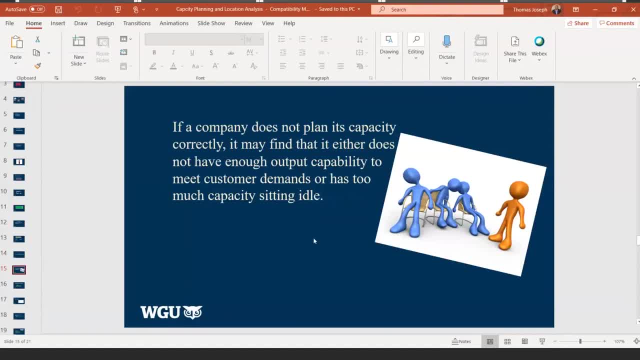 So if the organization does not properly plan its capacity, there is a high possibility that you have staff coming to work and they have nothing to do. They're just chilling. There is nothing to do. If you effectively plan your capacity, then your staff will always have a sufficient amount of work for them to do. 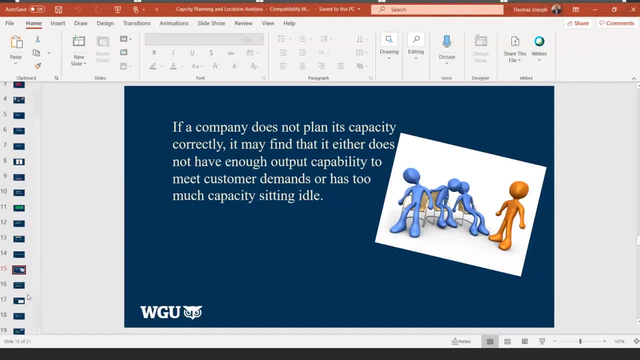 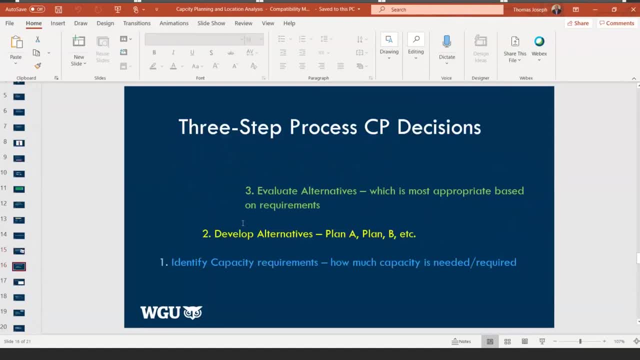 You will meet the production demands. You will meet your customer needs as well. So capacity planning, essentially, is important. So how does a manager, you as a manager, how do you follow and make capacity planning decisions? If this is important, then I have to have a process in place. 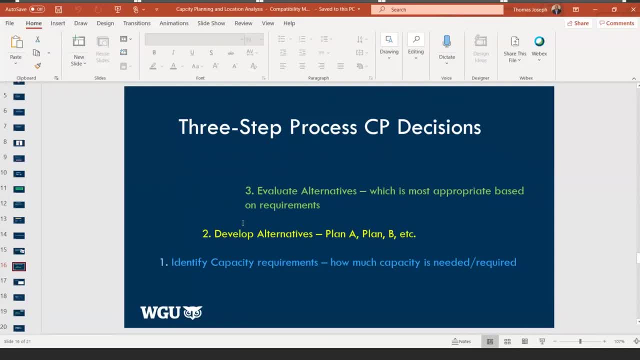 For me to make the right decisions, to plan out my capacity. So we start at the bottom. Step number one: identify capacity requirements. Again, remember that, how much capacity is needed, how much is required? Once you figure it out, then you develop an alternative. 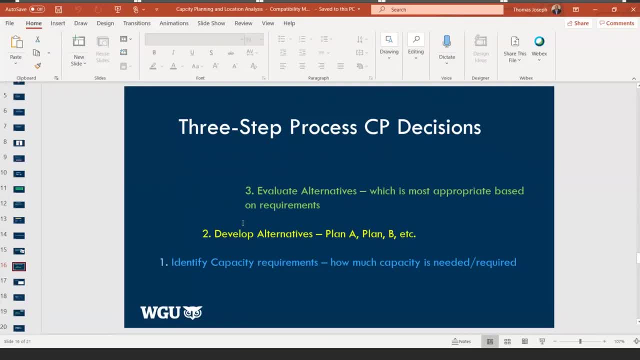 It's always good to have a plan A, a plan B, a plan C or a plan D, Because if plan A doesn't come to pass, then you can go with plan B And then, thirdly, evaluate alternatives, which is more appropriate. 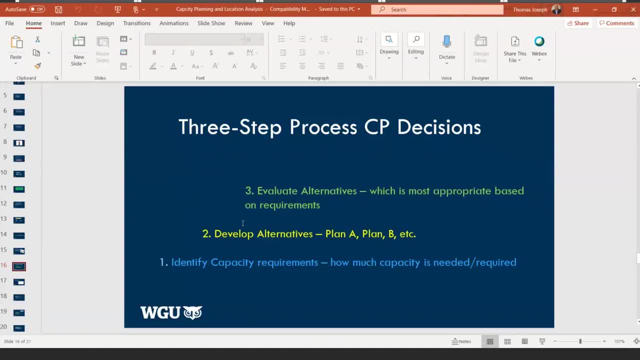 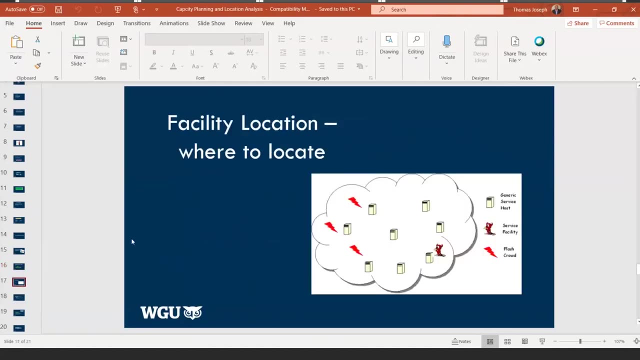 Based on the requirements. We do this all the time. If you're deciding to move, then these are the things that you do. How much space do we need? All right, should we go to the north or are we going south And then, based on that, based on what south has to offer, you decide which way you want to go. 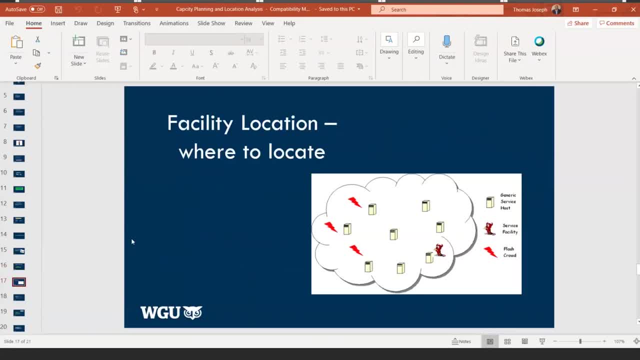 All right. so that brings us into facility location. Based on that decision making process, it brings us to where do we locate Right? If you are an aspiring business owner, you decide: one day I want to start my own business. this will come to play as well. 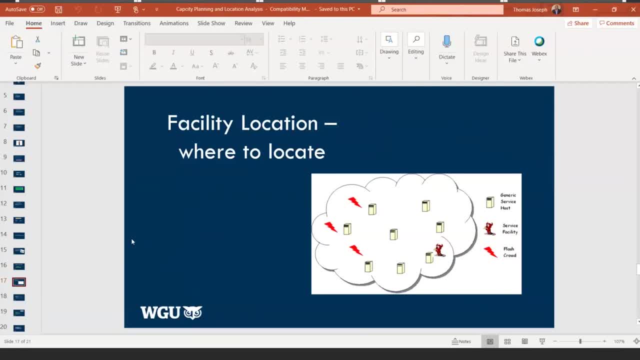 Because, now that you know how many clients you want to serve per day, per week, per month, per year, you want to decide: where am I going to put my business, Where am I going to locate? Where am I going to operate? 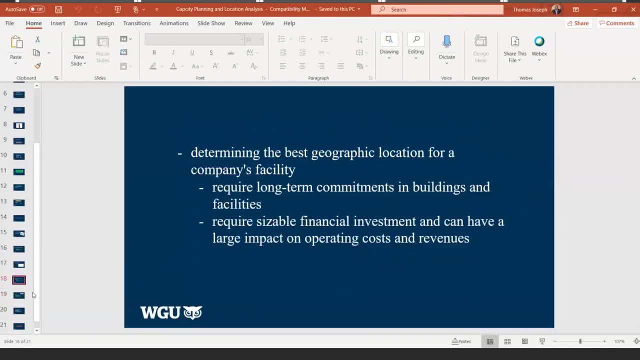 Right. So in facility location you determine the best geographic location for your company's building Or facility. That could require long-term commitments in buildings Right, Which could be costly, Or that could also require short-term commitments. It all depends on where you decide to locate and how long you want to be where you plan to be. 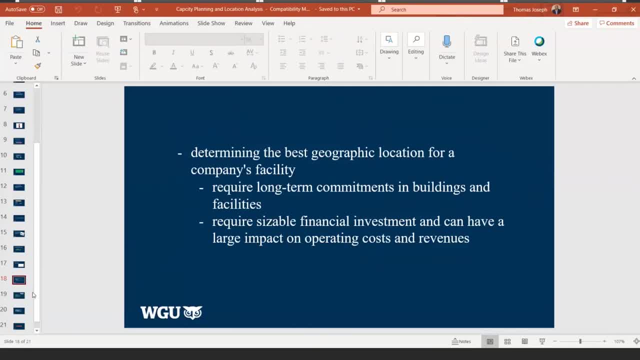 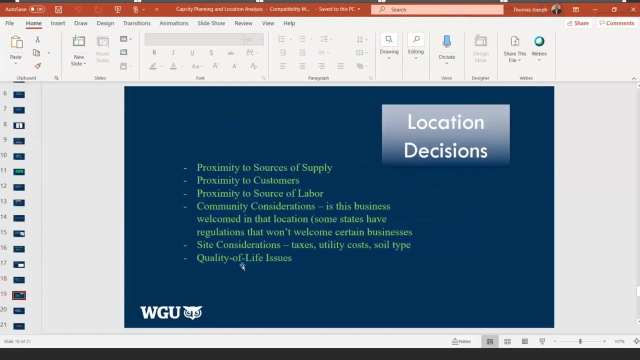 It also requires financial- sizeable financial investments- and can have a large impact on operating costs and revenues. So, taking those into consideration, Organizational managers have to ensure that they are making the right decisions on where to locate the organization. Where do we put our business? 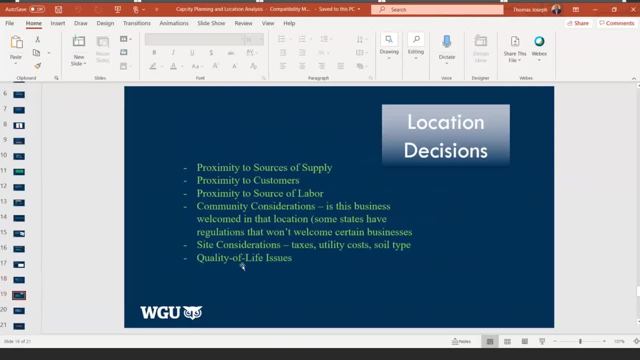 Where do we go and function and have our services available for customers? So here are some things or some factors that impact that decision. Right Number one: proximity to sources of supply Right. So let's say you are a business owner, Right. 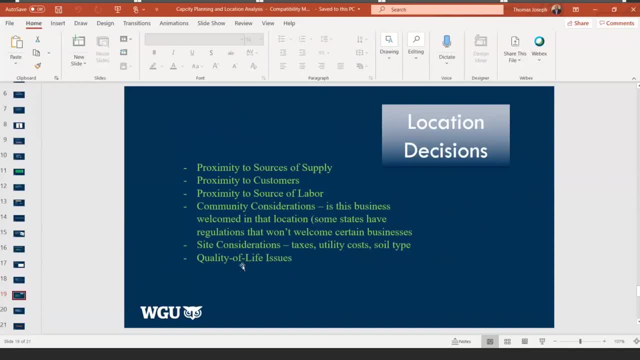 You decide to open like a grocery store, Right, How far will my grocery store be from the suppliers who are supplying groceries or products to me? If you are, I'm giving you guys big positions. You decide I am a. what can we come up with? 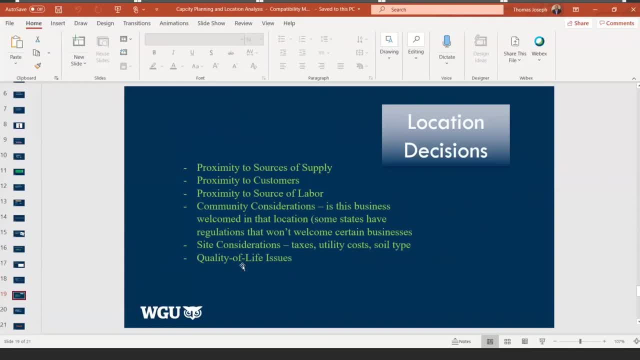 I'm into healthcare, So I'm going to start off my own physical therapy office. Right, I will have companies delivering machines Delivering machines to me and equipments that I need. How far do I want them to be from me, Right? 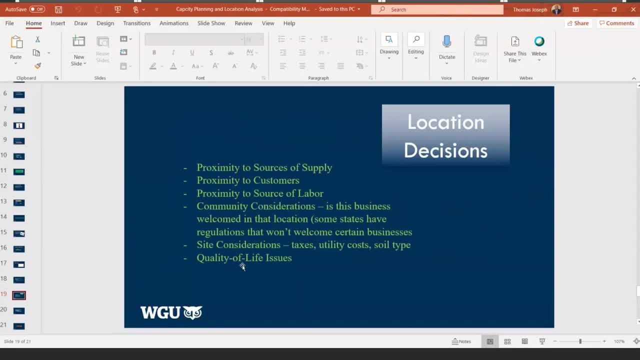 Am I going to locate in an area where it's going to take 20 miles, 20 hours for my suppliers to drop off supplies for me? I have to take that into consideration. Another thing to consider is proximity to customers. How far or how close do I want to be from customers? 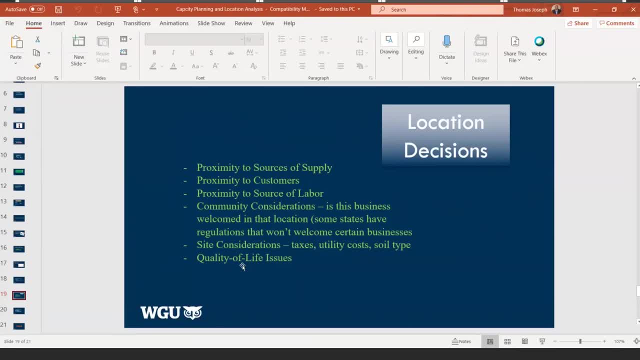 Proximity to sources of labor. Consider community considerations. Remember we talk about if you were to relocate. you build your family. Now you have a house of five instead of a house of one. Then you want to think of where do I want my kids to go to school? 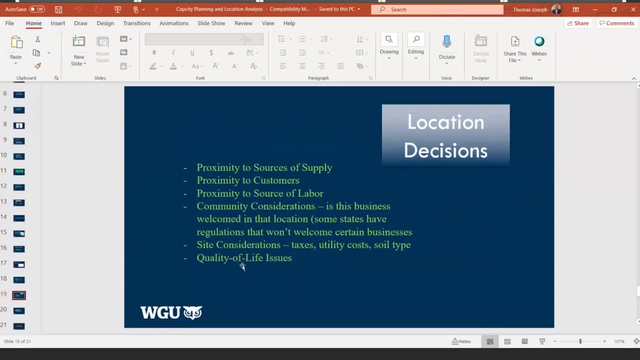 What type of neighborhood do I want to live in? I take all those into consideration. In a business perspective, it says: is this business welcome in that location? Some states have regulations that would welcome certain businesses. I remember living in a town, in a state, in a certain state, and they would not welcome casinos. 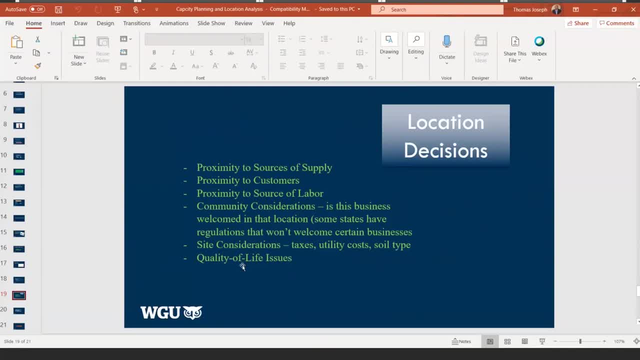 Casinos were not welcome into those places, So nobody could open a casino there. Another factor that impacts location decision is site considerations. We can think in cases of taxes, utility costs as far as the soil type And, last but not least, the quality of life issue. 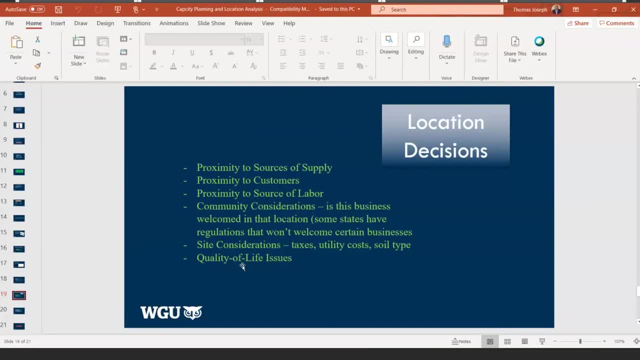 That is, remember. every business has a responsibility to its community, Right. It has a responsibility to the environment as well. So is that service going to provide a quality of life to the people that you're going to serve? And all of these questions, or all of these factors, have to be taken into consideration. 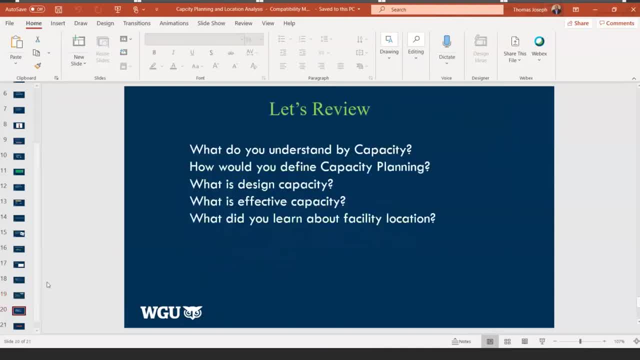 before an organization can make that decision to say: okay, we're going to locate here, or we're not going to locate here. We're going there, or we're not going there, All right. So here are some things based on our discussions for you guys to take into consideration. 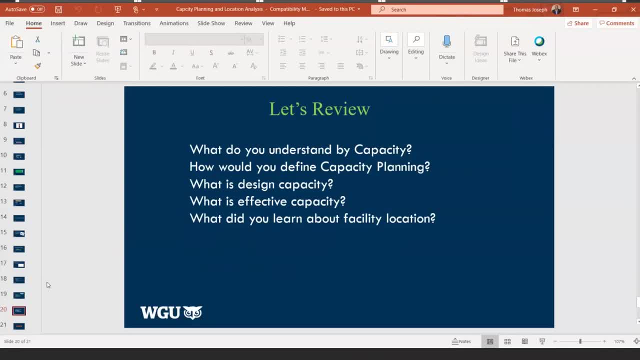 as you consider the idea of capacity, capacity planning and also location decision. What do you understand by capacity? Here are some things to think about. Recapping on the things that we talk about. What do you understand by capacity? Remember, it's a maximum output. 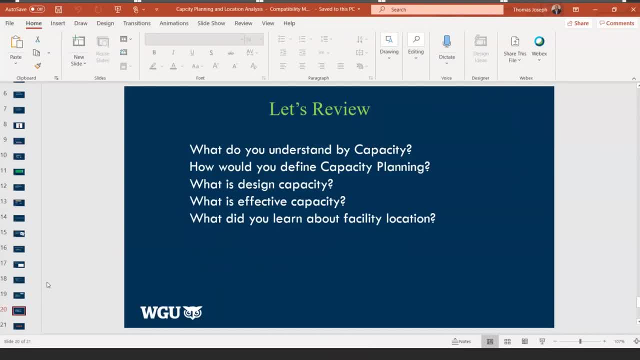 How would you define capacity planning? We have the maximum output. We know how much capacity we need, where we need capacity. Now we have to make that plan and put some actions into perspective to decide where business should be located. How should we function? 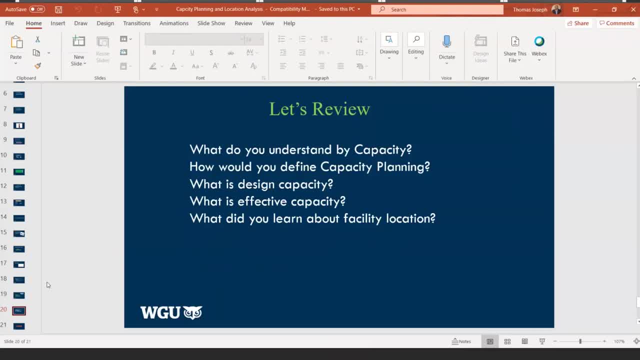 How many employees do I need to have in today? How many do I need not to have it? And then, what is this? What is the design capacity? What is effective capacity And what did you learn about facility location? Here are some concepts. 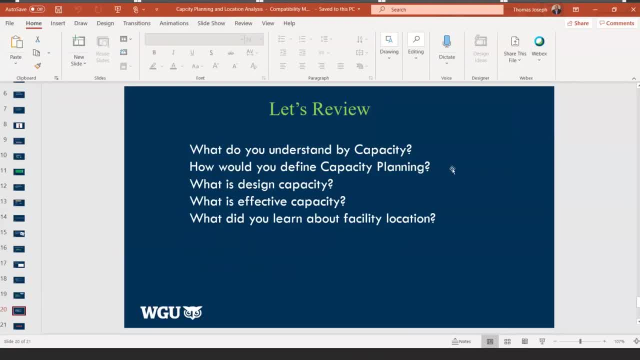 Here are some thoughts for you to think about as we explore and as you review and explore the concept in the text as well, based on capacity.